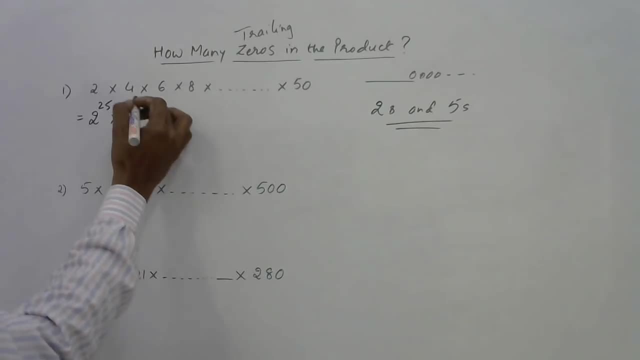 2 divided by 2 is 1.. 4 divided by 2 is 2.. And what is left is: 2 divided by 2 is 1.. 4 divided by 2 is 2.. 6 divided by 2 is 3.. 4 divided by 2 is 4.. And so on. up to 50 divided by 2 is 25.. In this series, 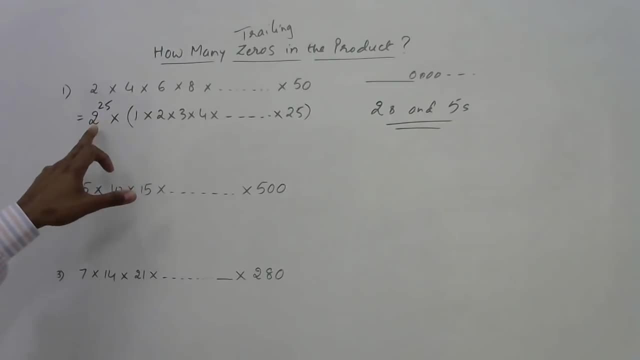 we have enough number of 2s. So 2 raised to power 25 means 25 2s are already there and here also we have some 2s. So let us find the number of 5s here first. So 2s are enough more And 5s are. 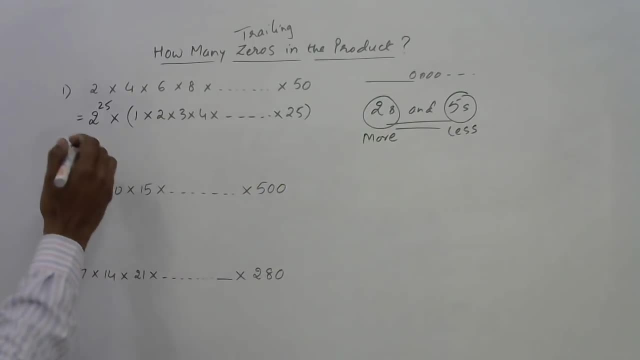 less In this series. My intention is to find the ones which are less, So let us find the number of 5s. Number of 5s. How do you find the number of 5s? How many terms are there? 25.. So 25. 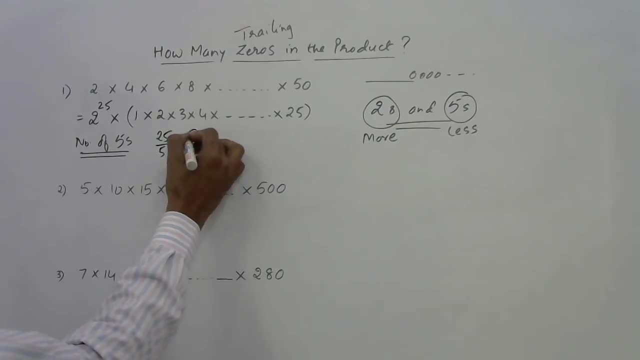 divided by 5 is 5.. And further 5,. this quotient divided by 5 is 1.. Now 1 cannot be divided by 5.. So number of 5s is 5 plus 1, 6. Number of 2s is far more than 6. That is 25 plus. Some of the 2s are here also. 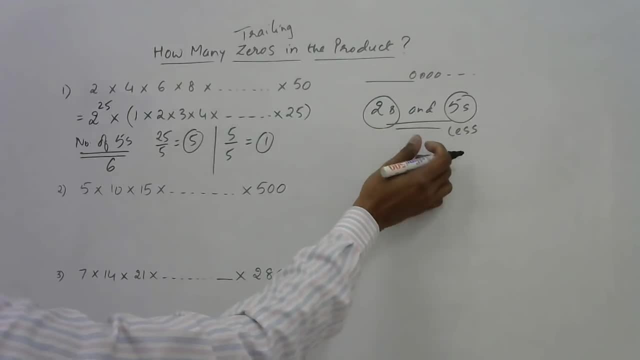 So you can write for this question: how many 2s are there? 2s are more than 25.. And 5s are only 6. So which of them are less Less is 6.. So number of 0s in this question will be 6.. 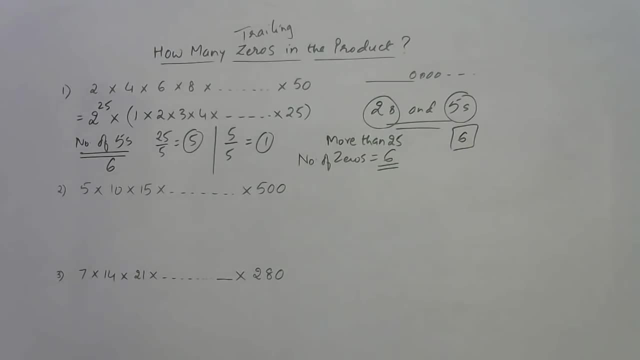 If you have understood this well and good. If you have not understood, let us take up 7.. Now see for 7, we have 7 into 1,, 7 into 2, 7 into 3, up to This is 7 into 40. So 7 raised to power, 40 will be there outside. 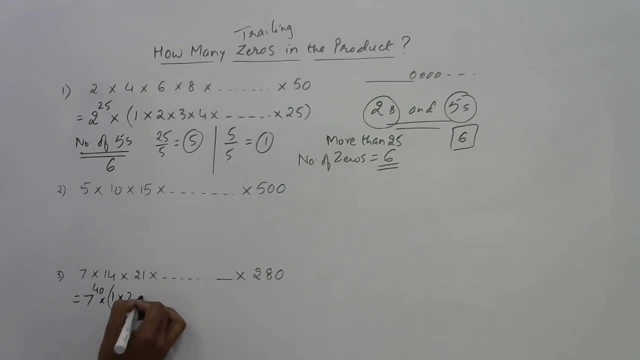 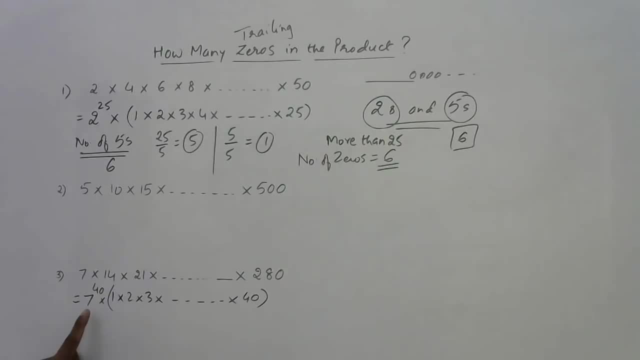 Now 7 raised to power 40 will have all 7s 40 times. So just neglect this. 1 to 40, we can test how many 2s and how many 5s. So for 2s, 40 divided by 2 is 20.. Then 20 divided by 2 is 10.. 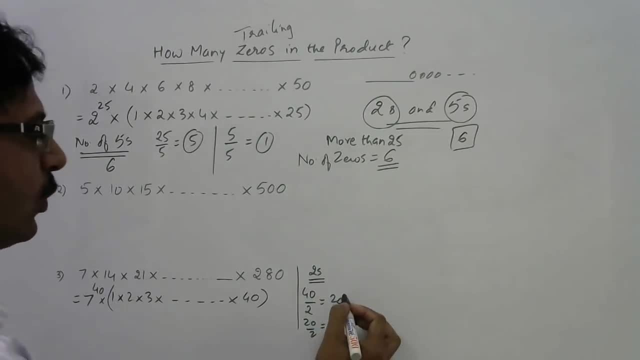 And so on. So number of 2s will be more than 30.. But what about 5s? Last term is 40.. So 40 divided by 5 is 8.. And 8 divided by 5 is 1 quotient and 3 remainder. 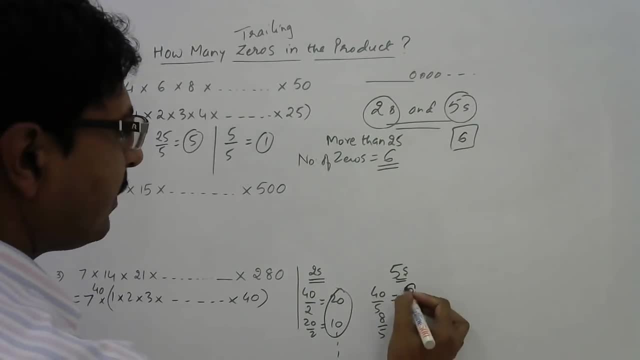 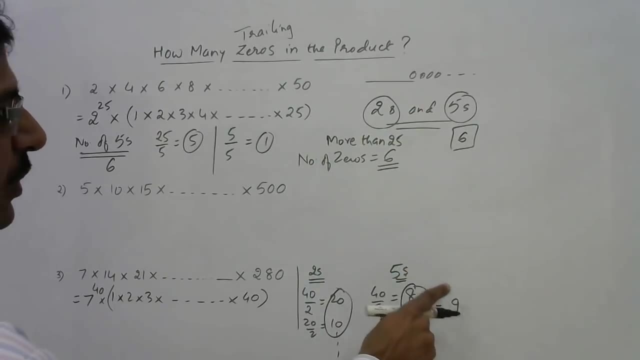 Now, 1 cannot be divided by 5.. So 8 plus 1,, 9, 5s in this product. So 2s are more than 30 and 5s are only 9.. So we have to consider only the one which is less. 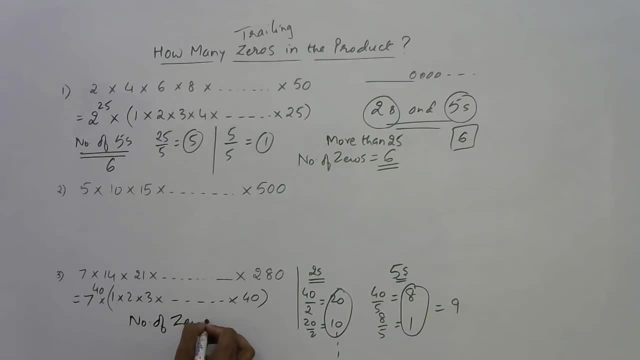 So number of 0s in this case will be 9.. Likewise in this case, see, this is 5 into 1,, 5 into 2,, 5 into 3, up to 5 raised to power, This is 5 into 100.. So 5 raised to power, 100 will come outside. 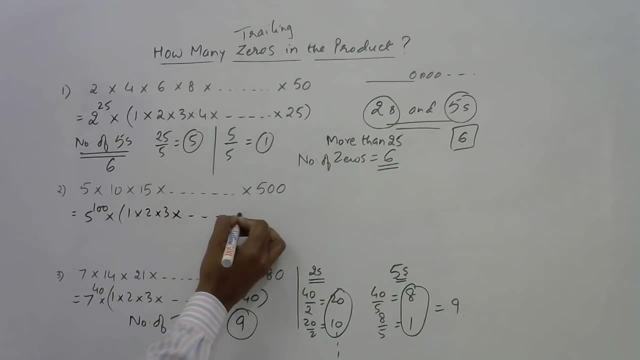 And you will have 1 into 2 into 3, up to 100.. Now see: 5 raised to power, 100 will come outside. 5 raised to power 100 will come outside. In this case, 5s are at least 100 here, plus some 5s here also. 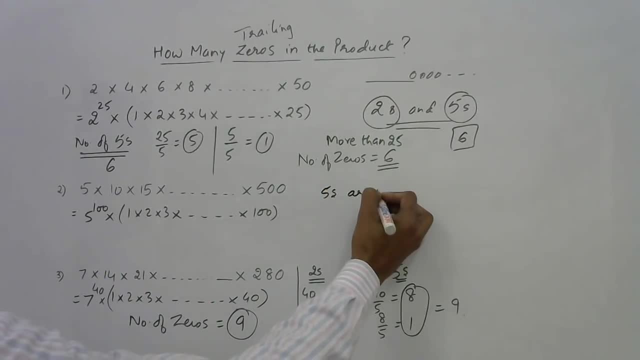 So I can see that 5s are more in number, So I just leave 5.. So I need to find out 2s. For finding the 2s, this is 100.. 100 divided by 2 is 50.. 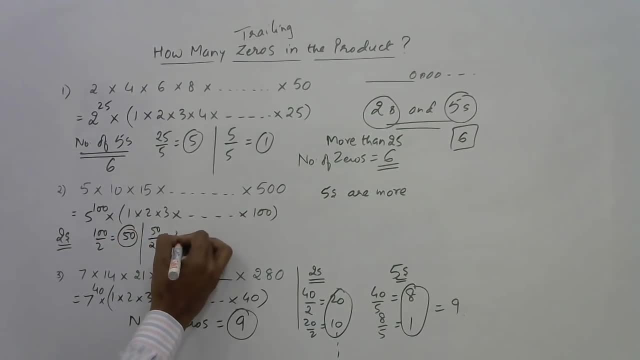 50 is more. So 50 divided by 2 is 25.. 25 divided by 2.. Just leave the remainder. Just take the quotient: 25 divided by 2 is 12.. And 1 remainder, just leave the 1.. 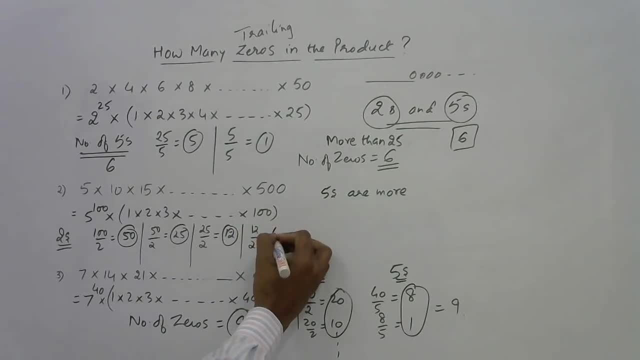 Further: 12 divided by 2 is 6.. 6 divided by 2 is 3.. 3 divided by 2 is 1.. Now see, we cannot divide further. So how many 2s are here? 2s is equal to just add. 50 plus 25 is 75..